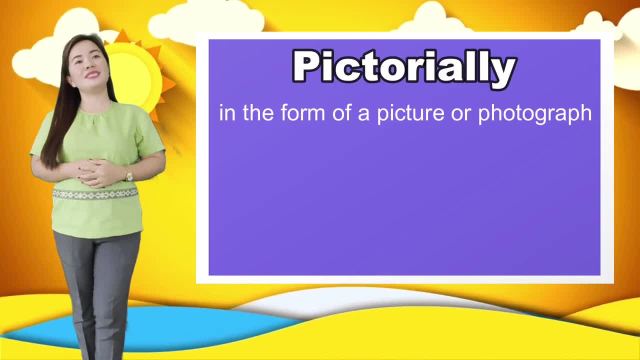 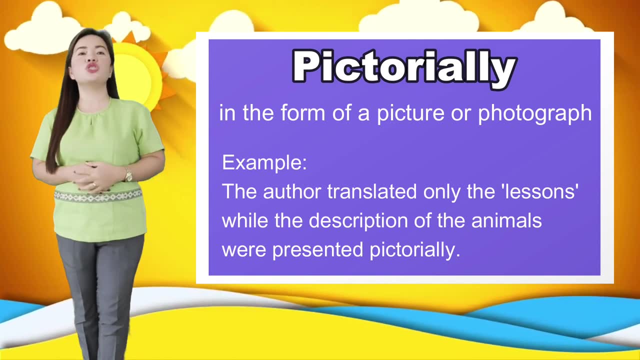 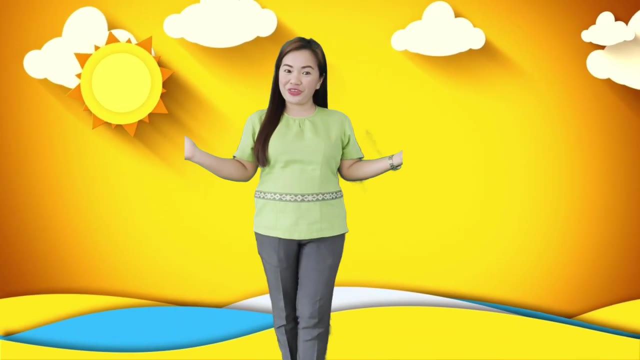 Number 3, Pictorially Means in a form of picture or a photograph. Example: the author translated only the lessons, while the description of the animals were presented pictorially. So without further ado, may I begin my story about Ravindra, who is strolling and found three brothers. 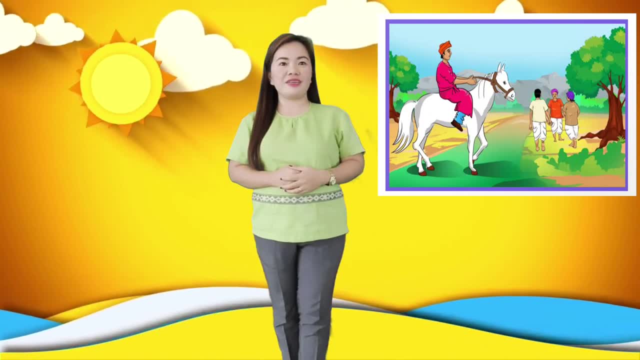 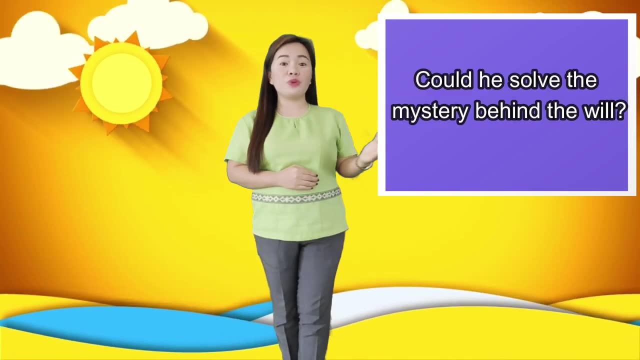 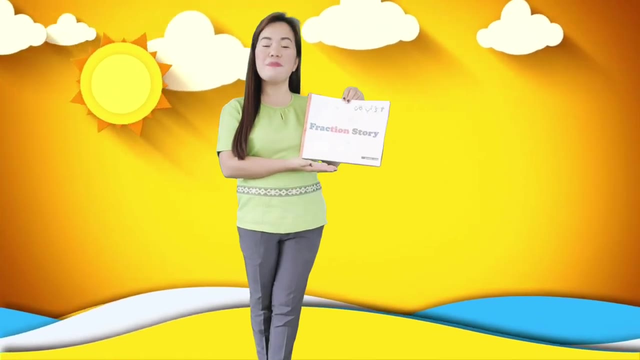 puzzled with a strange wheel in a form of rhythm. He understood that he had to apply math concept in the puzzle. Could he solve the mystery behind the wheel? This story is about fraction. Once there was a wise man, Ravindra. 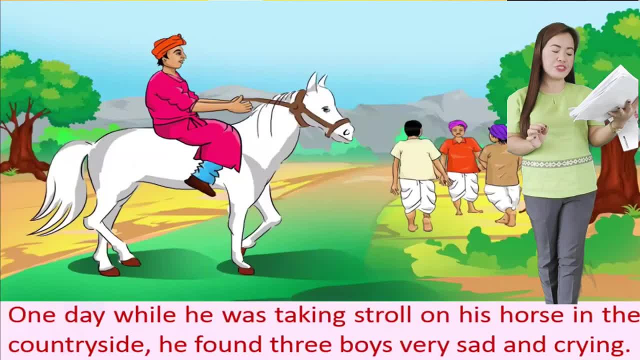 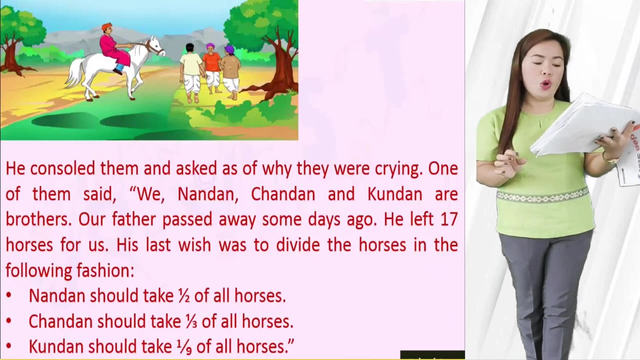 One day, while he was taking stroll on his horse in a countryside, he found three boys very sad and crying. He consulted and asked as of why they were crying. One of them said We, Nandan, Chandan and Kolban are brothers. 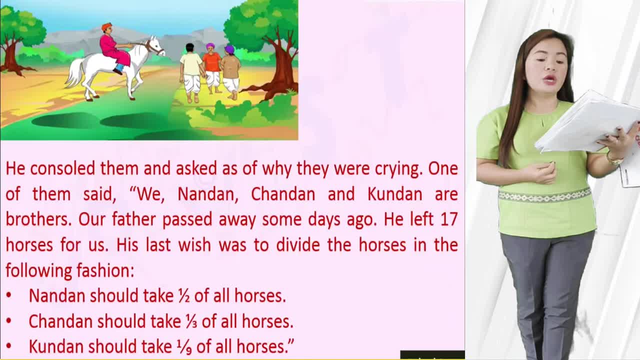 Our father passed away His mother, Lacey Ball, who led 17 horses for us. His last wish was to divide the horses in the following fashion: Nandan should take one half of all horses. Chandan should take one third of all horses. 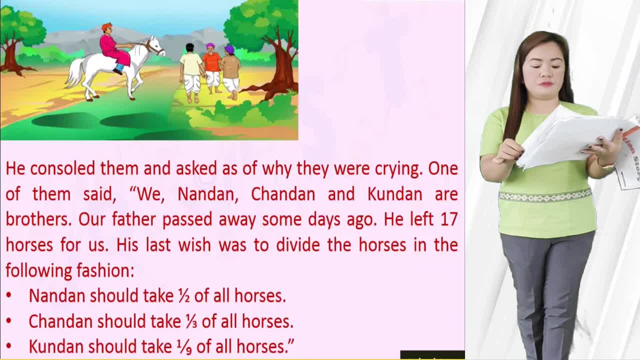 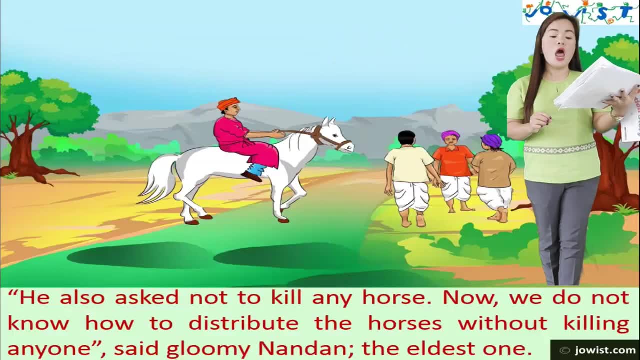 Kondan should take one ninth of all horses. He also asked not to kill any horse. Now we do not know how to distribute the horses without killing anyone. Sad, gloomy Nandan. the eldest one, Chandan, spoke then. 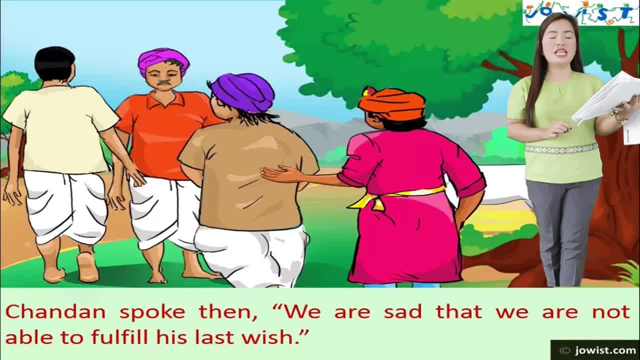 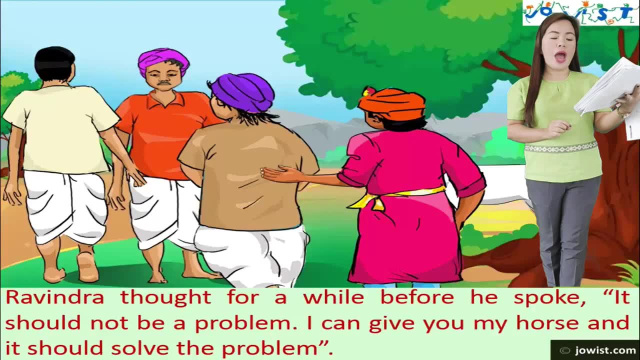 We are sad that we are not able to fulfill his last wish. Ravindra thought for a while before he spoke. It should not be a problem. I will give you my last wish. I will give you my last wish. It should not be a problem. 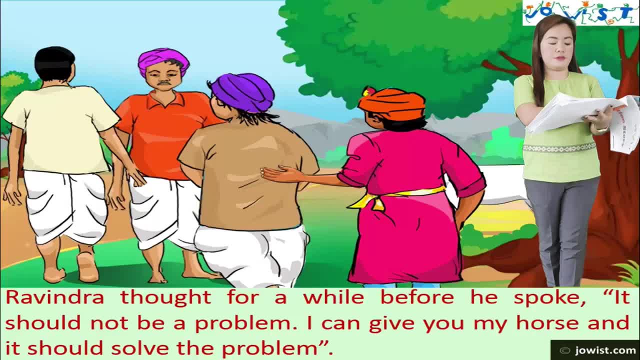 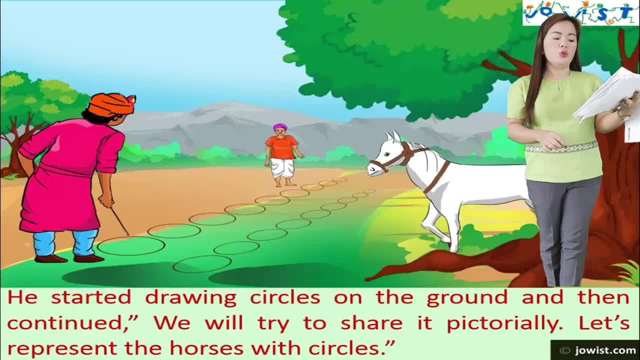 I will give you my last wish. I will give you my last wish. This is my worst and it should solve the problem. He started drawing circles on the ground and then continued. We will try to share it pictorially. Let's represent the horses with circles. 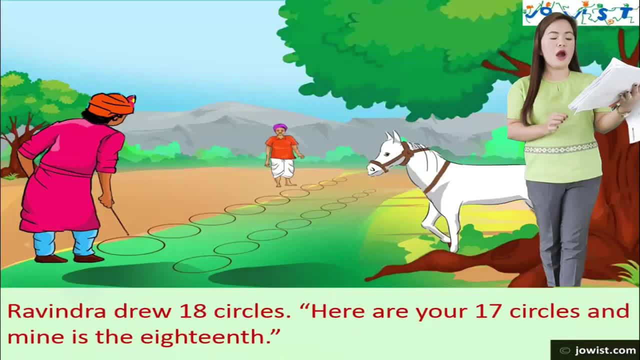 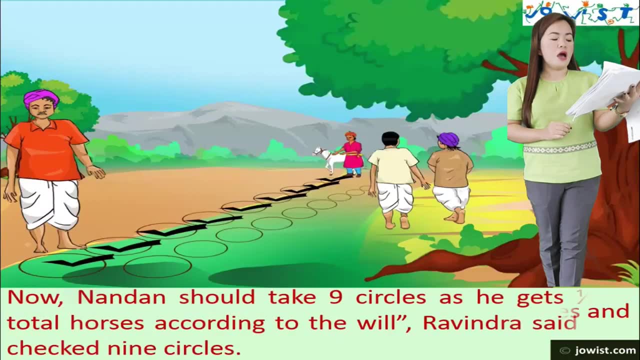 Ravindra draw 18th Circles. Here are your second two circles and mine is the 18th. Now Nandan should take nine circles as he gets one half of the total horses according to the wheel. Ravindra said and checked nine circles. 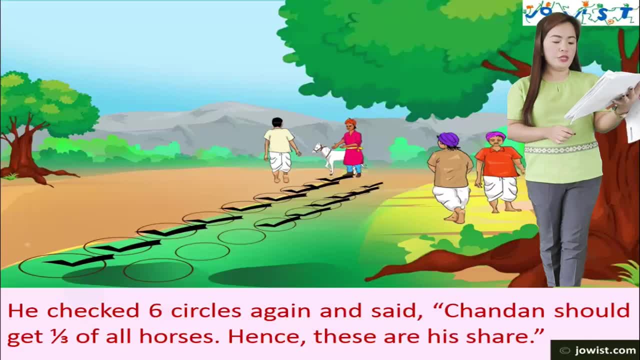 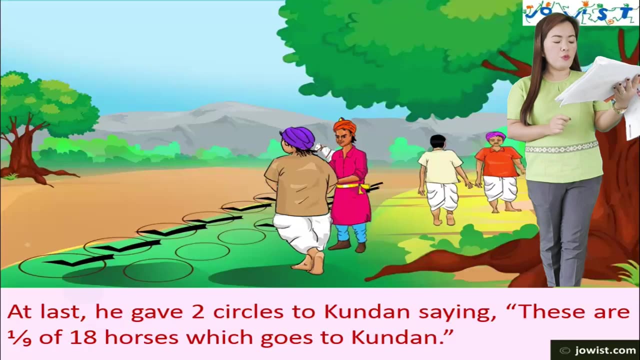 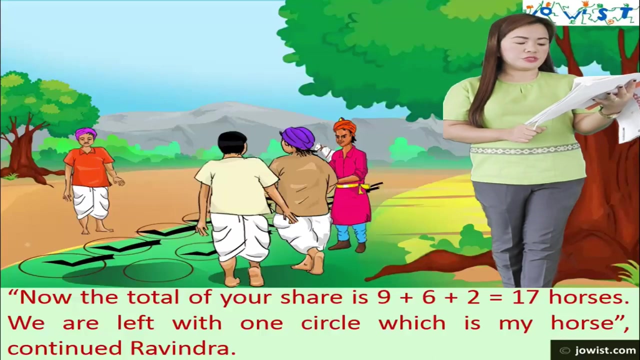 He checked six circles again and said Chandan should get one third of all horses, hence these are his share. At last he gave two circles to Chandan, saying These are one ninth of eighteen horses which goes to Chandan. Now the total of your share is nine plus six plus two equals seventeen horses. 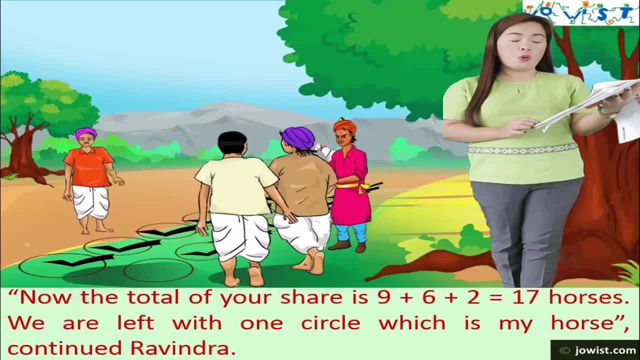 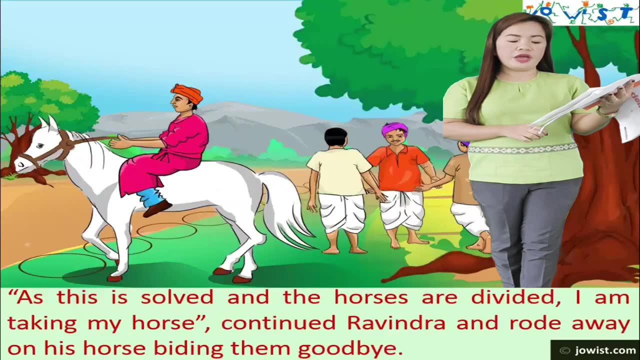 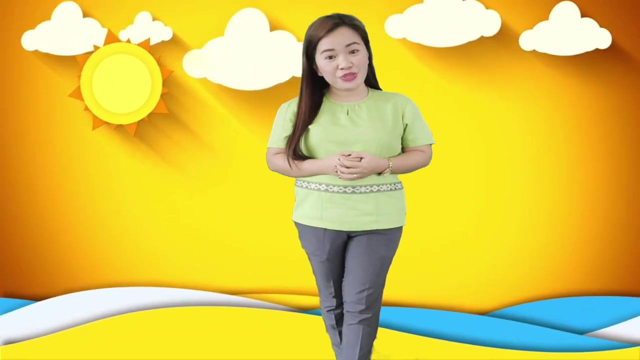 We are left with one circle, which is my horse, continued Ravindra. As this is so and the horses are divided, I am taking my horse, Continued Ravindra and rode away from his horse, biding them goodbye. Did you enjoy the story I've shared with you? 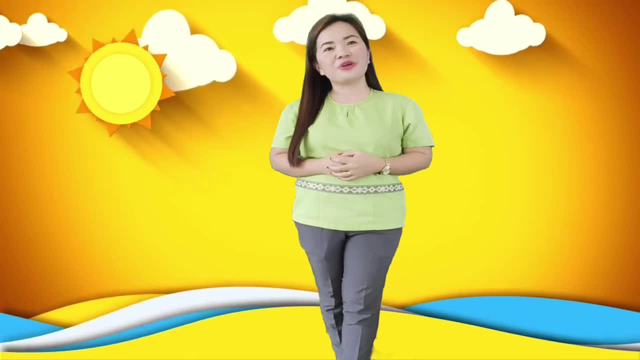 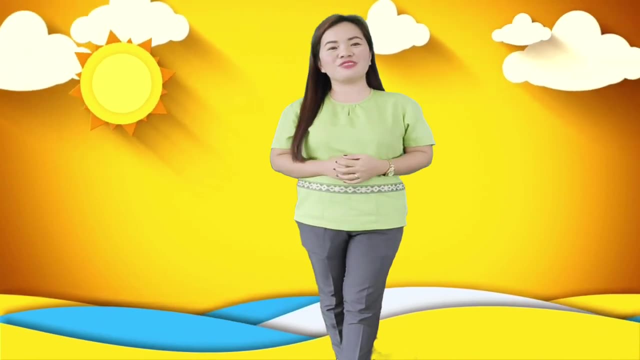 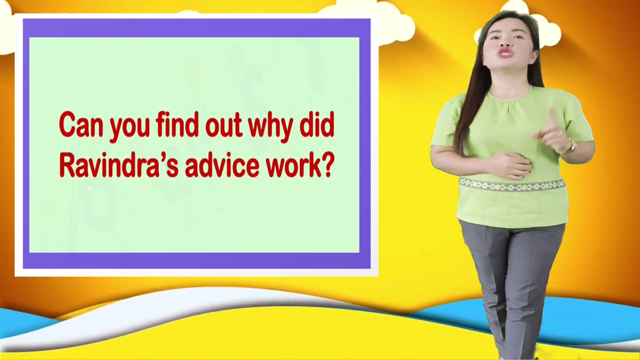 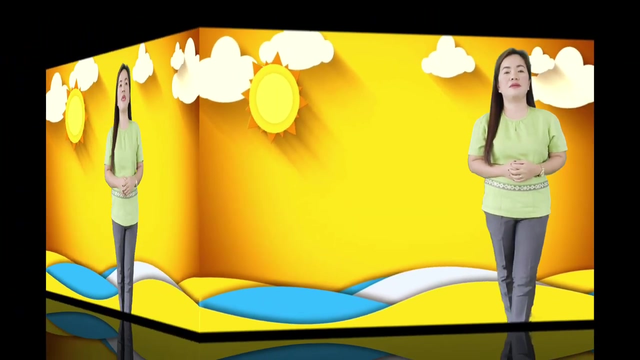 Great, I am happy that you enjoy and learn something from the fraction story you've listened earlier, So I have a questions for you to think about. Can you find out why did Ravindra's advice work? So please write your answer on the chat box so that I may be able to read your answer. 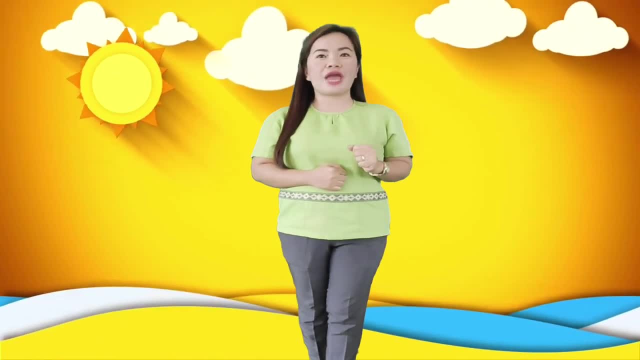 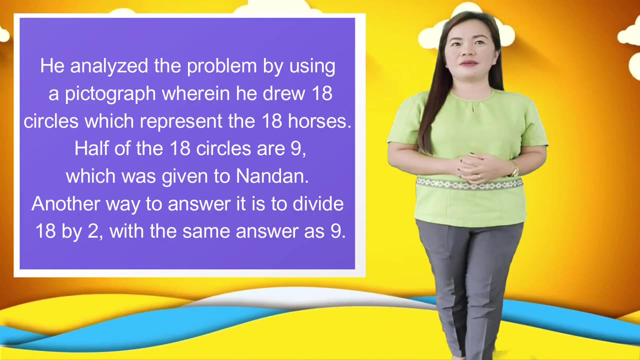 Excellent answer kids. Ravindra's advice worked because they were able to divide the inheritance of the three brothers as what had been asked by their father before he died. This is what Ravindra did. He analyzed the problem by using the pictograph. 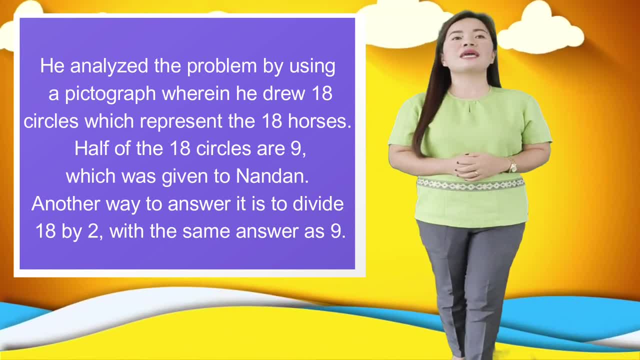 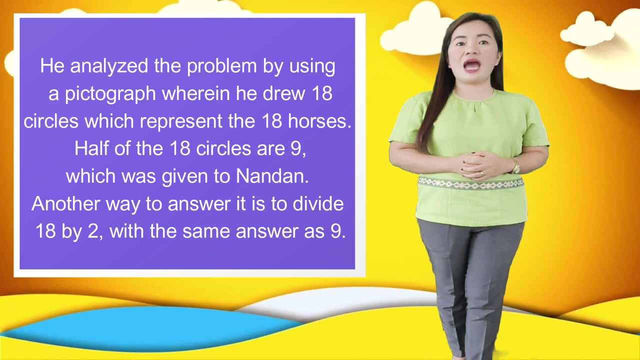 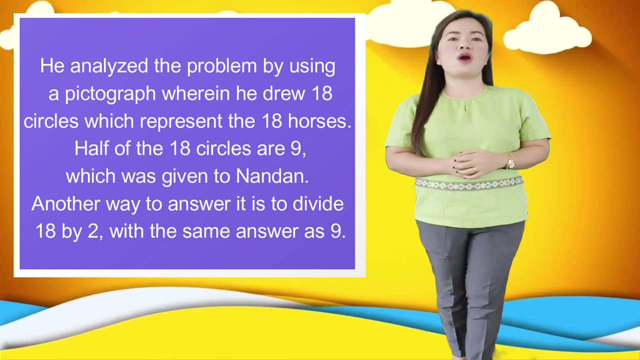 He drew 18 circles which represent the 18 horses. Half of the 18 circles are 9, which was given to Nandan. Another way to answer it is to divide 18 by 2, with the same answer as 9.. One third of the 18th circle is 6, which is given to Chandan.